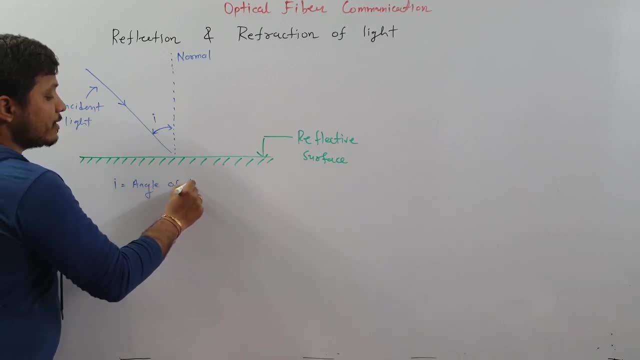 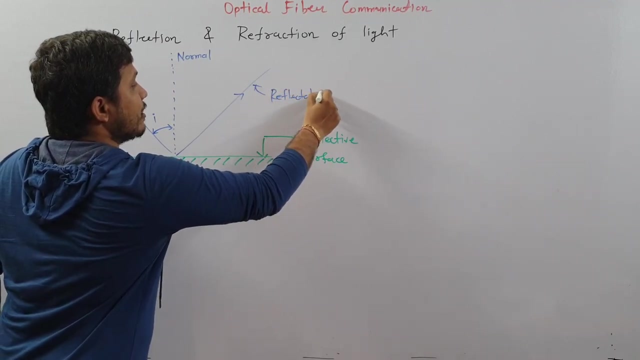 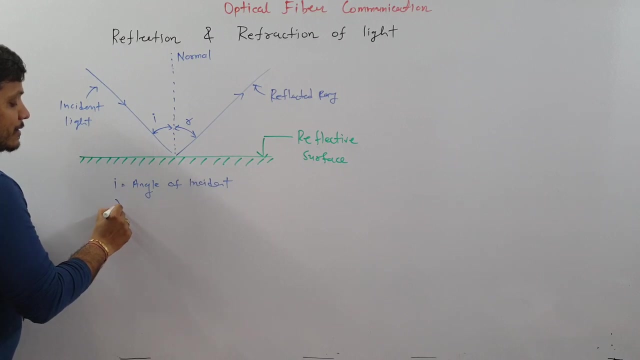 angle of incident. So when ray of light is getting incident on a reflecting surface, it will get reflected from that surface and this is what a reflected wave, reflected ray or wave right, And if you see this angle, So this angle is angle of reflection, So R is angle of reflection and for reflection phenomenon, these both angles. 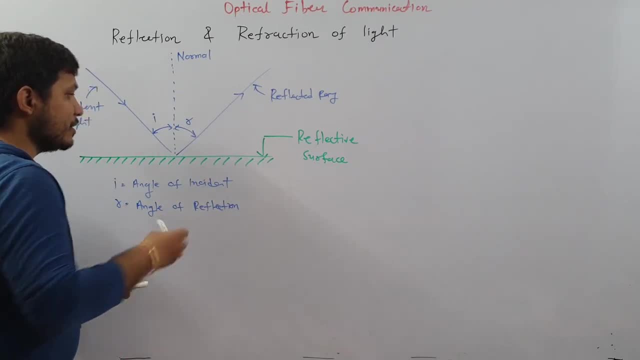 are same. So one can say: for reflection phenomenon, I is equals to R. So for the case of reflection, angle of incident and angle of reflection is same, it is equal. So this is how reflection is happening. Now see, let us try to understand how refraction happens. So in case of refraction, 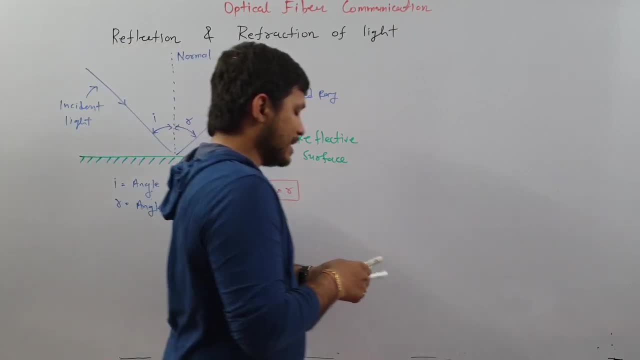 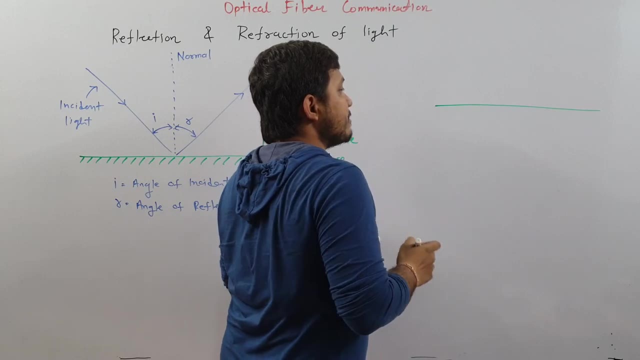 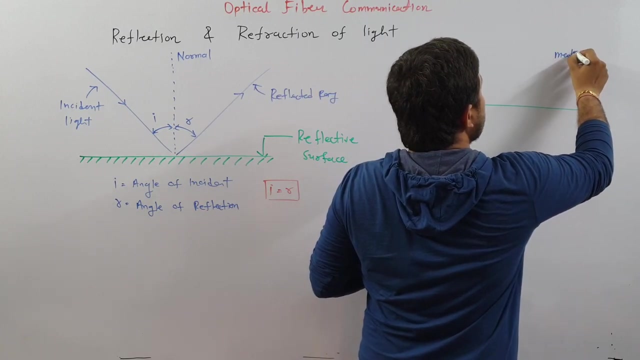 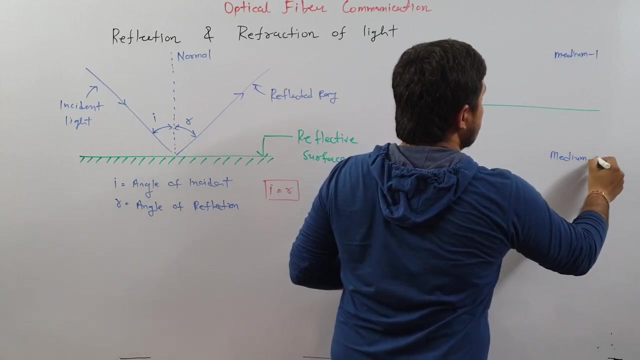 there are two things which is happening, So let us try to understand that. So if I say we have two mediums- and by this line I am separating two mediums- Here we have medium one and here we have medium 2, and let us have a ray which is getting incident. 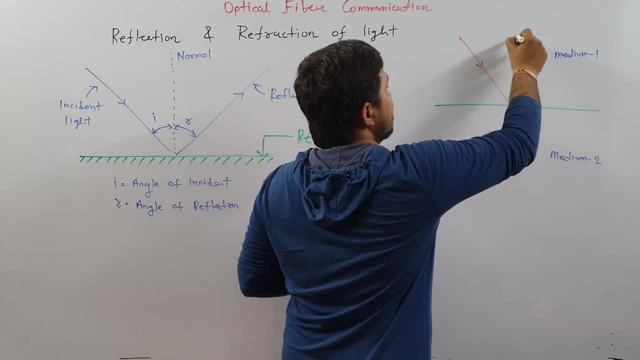 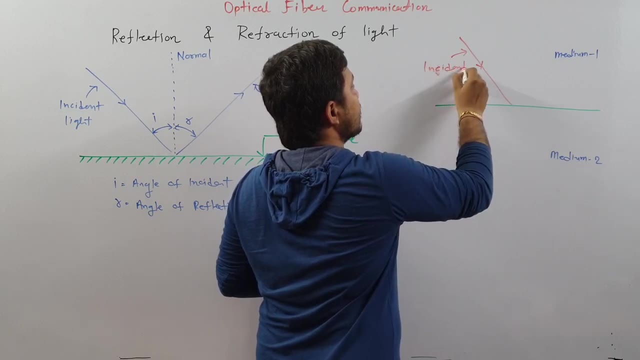 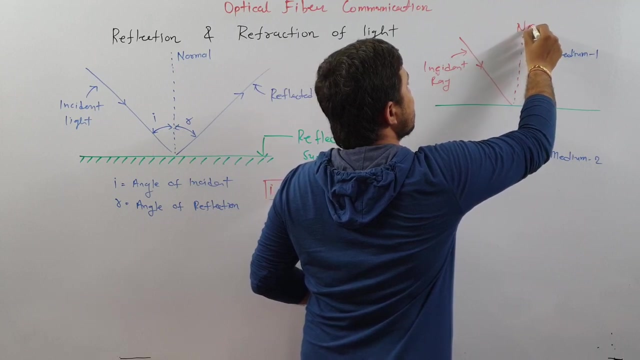 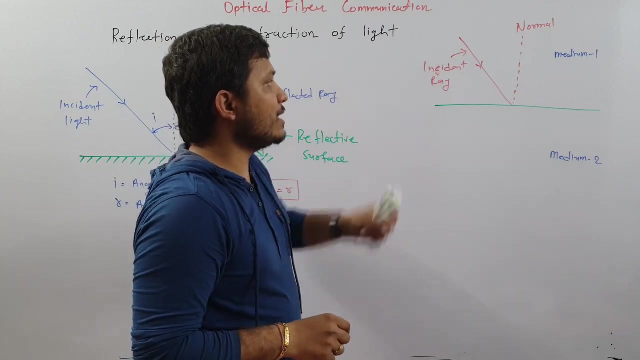 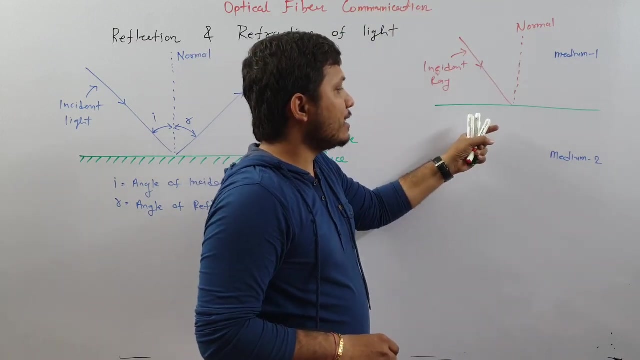 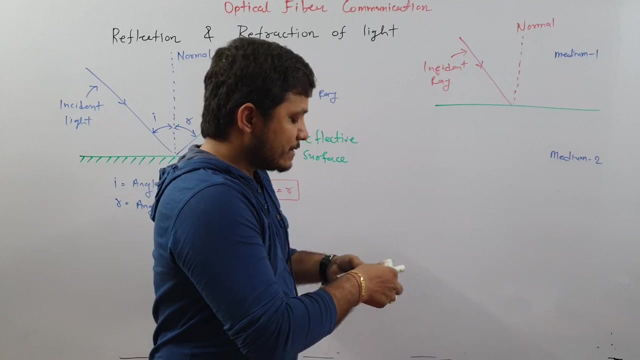 over here to the surface. so this is what incident ray and this is normal to the surface. now, here, if you observe, we have incident ray and this ray is entering from medium 1 and at the surface now it will get enter into medium 2. and if I say 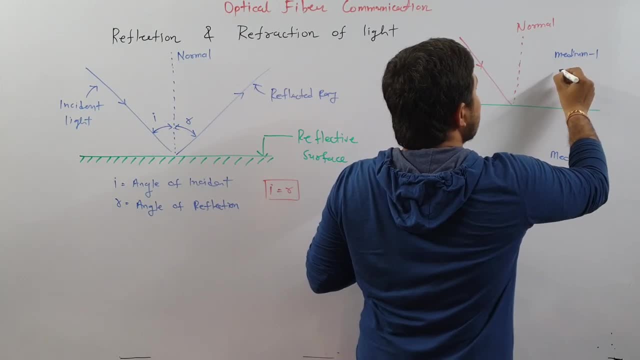 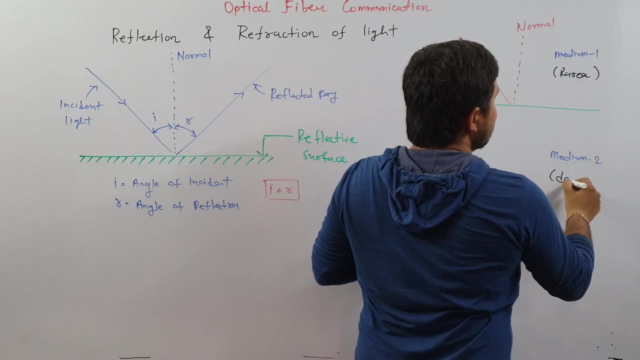 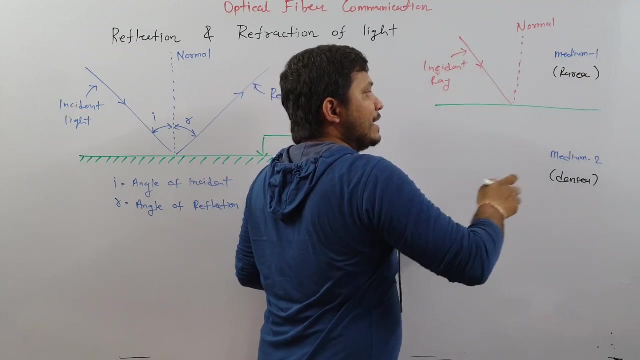 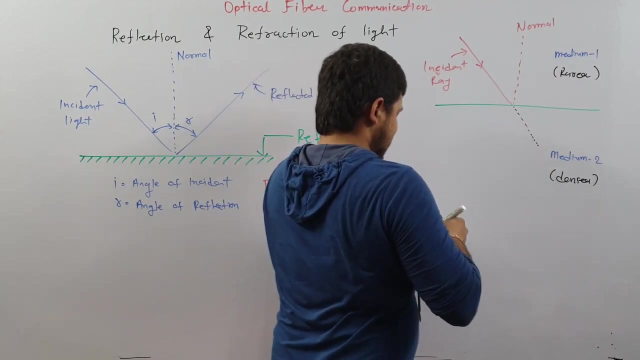 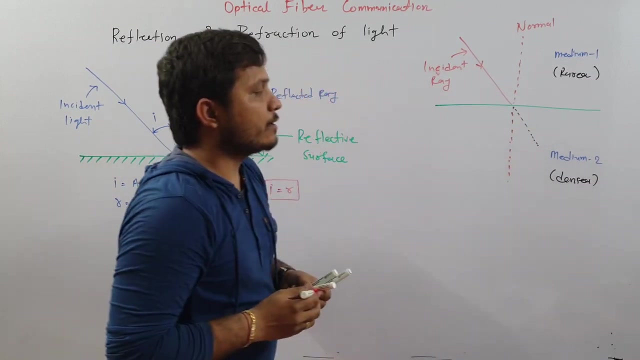 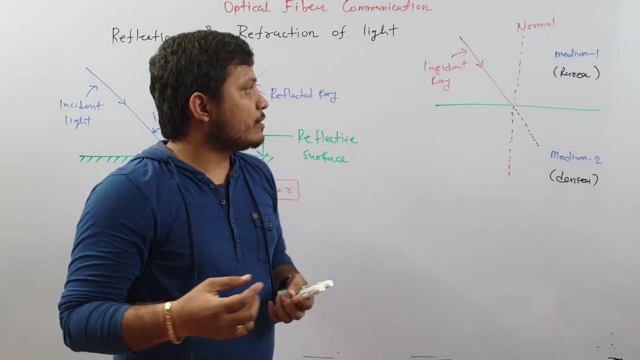 here medium 1, that is rarer medium, and medium 2, that is denser medium. so if you see this light, so its actual trajectory is this. this is what actual trajectory and here, this is what normal to the surface right now. when light enters from rarer medium to denser medium, at that time that light will get tilt, and what? 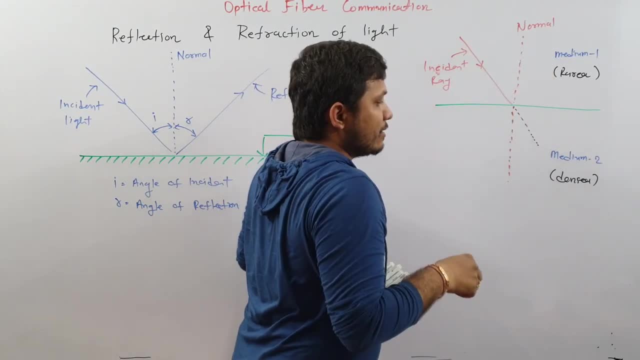 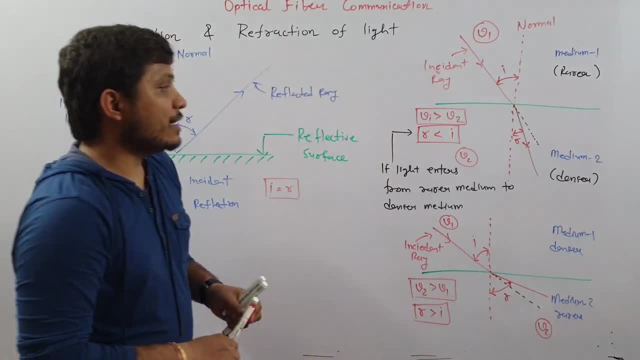 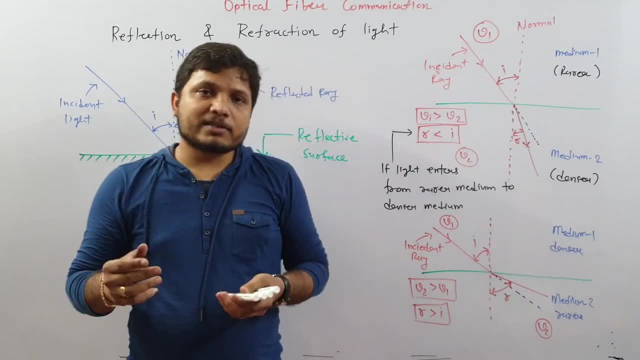 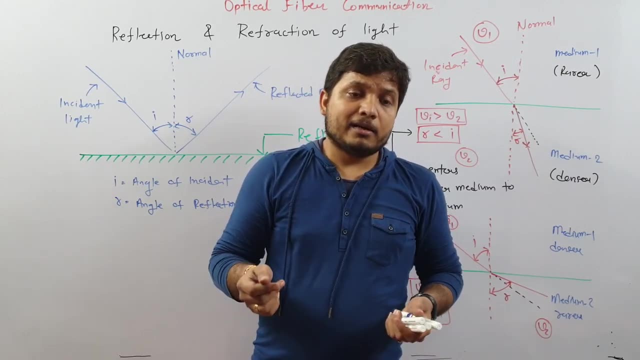 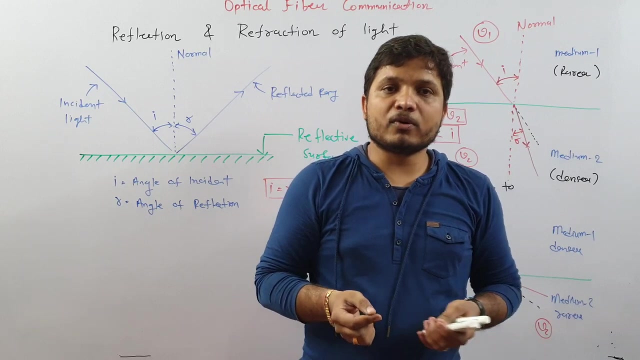 so, ultimately, what is refraction? so refraction is a phenomenon where, when light enters from one medium to other medium, that light is getting tiled, or one can say that light is getting banned, so that bending of light when it enters from one medium to other medium is called as refraction, and when light is getting, 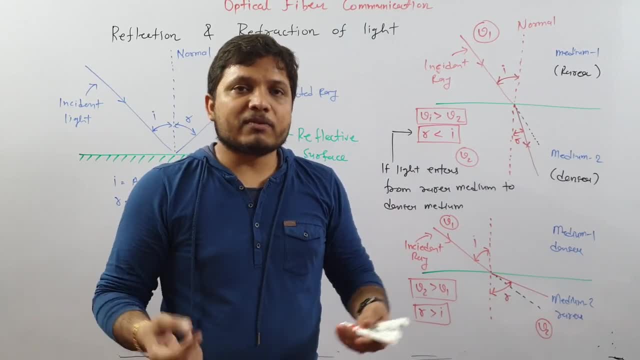 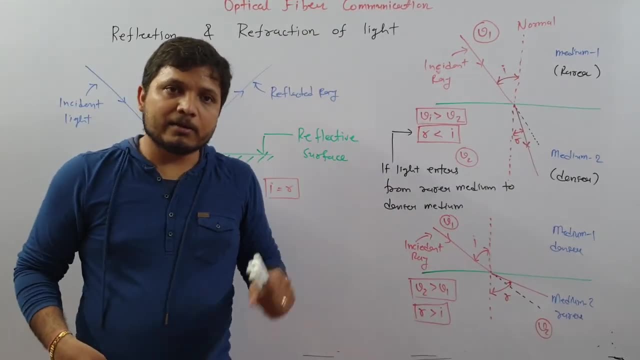 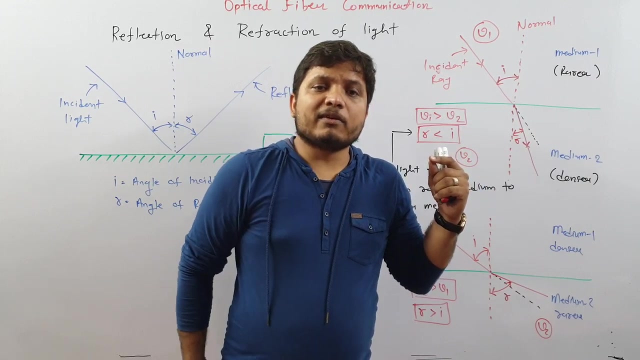 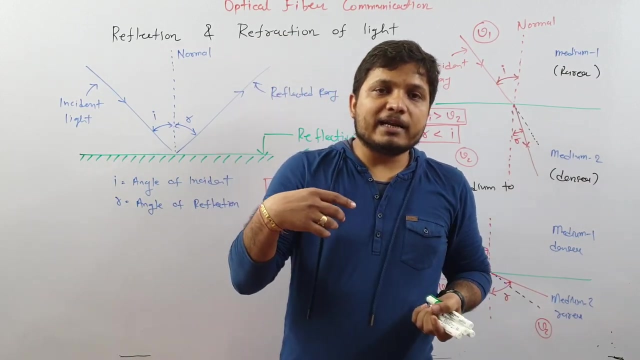 reflected from refractive surface. one can say: that is what phenomenon of reflection. In case of reflection, angle of incident and angle of reflection is same, while in case of refraction, one can observe angle of incident and angle of refraction. both are different and here you will be observing that angle of incident that will be greater.